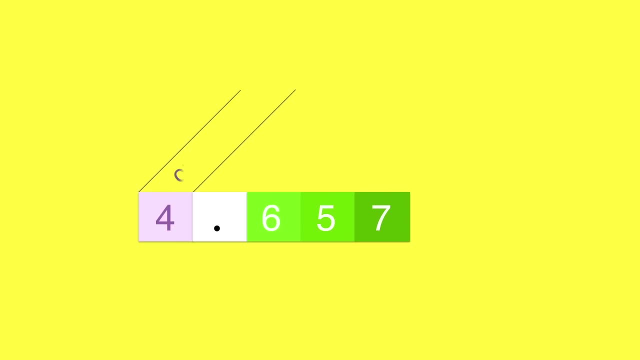 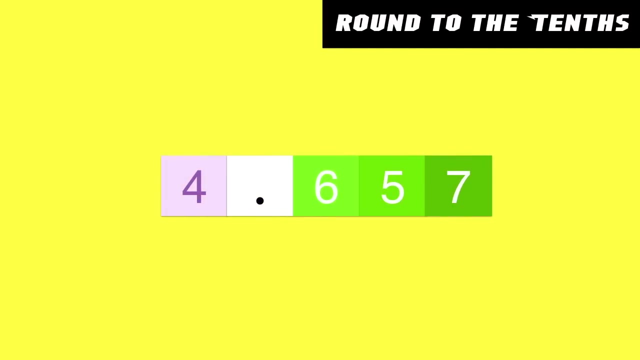 Welcome to rounding decimals. We already know that each digit has a number place with a place value name. You will usually be asked to round to a specific place value, like the tenths or the ones. First, let's try rounding a number to the tenths, Since we are rounding, 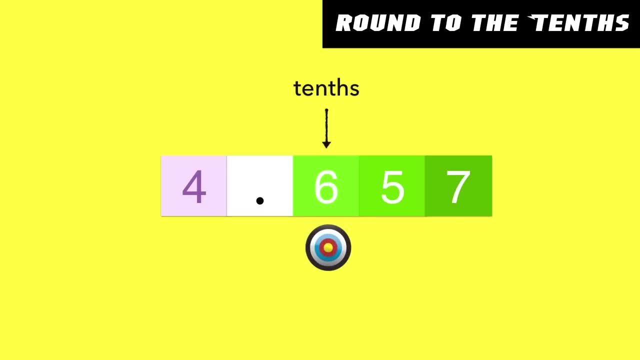 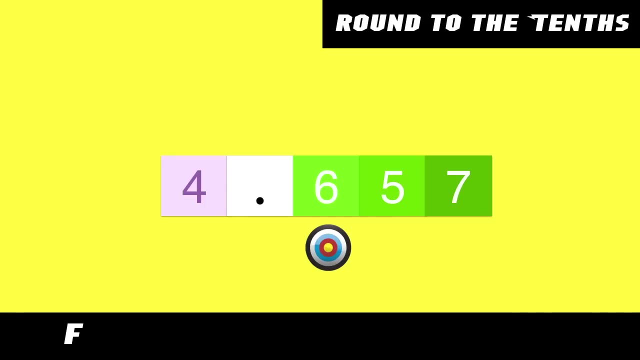 to the tenths. the tenths place becomes our rounding target. For rounding, I like to use a catchy rhyme: Who's that knocking on my back door? Five or more, raise the score. Four or less, leave that mess. Let's start from the beginning of the rhyme: Who's that knocking? 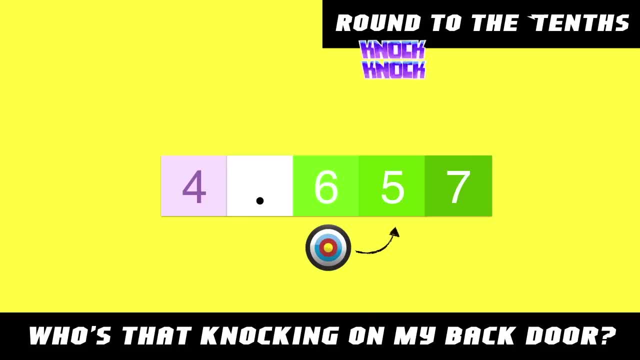 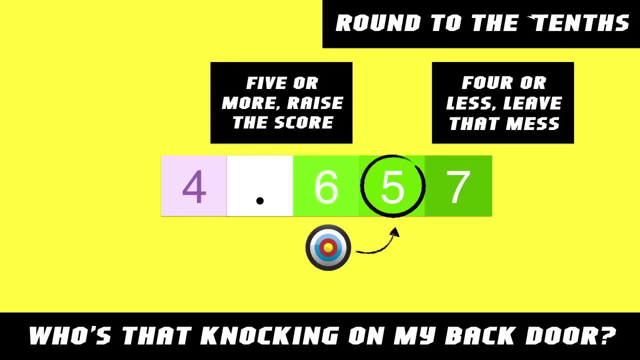 on my back door. When we look at the number placed behind six, we see that it is a five knocking. So will a five qualify as four or less? leave that mess, or five or more? raise the score. Five or more is correct, since the number knocking on the back door is five. Remember. 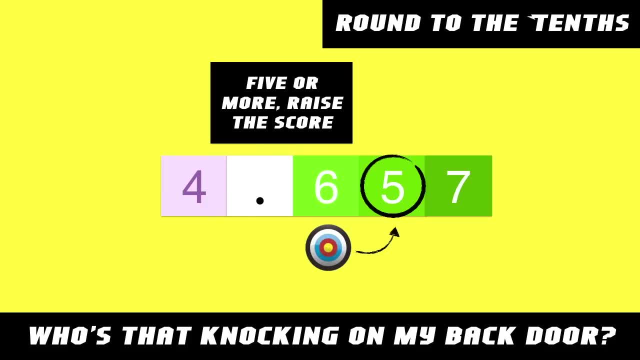 we're rounding to our target number. so what would six rounded up or raise in the score be? The six becomes a seven rounding up one. The place values to the right of the target number always become zeros and the numbers to the left of the target number always remain. 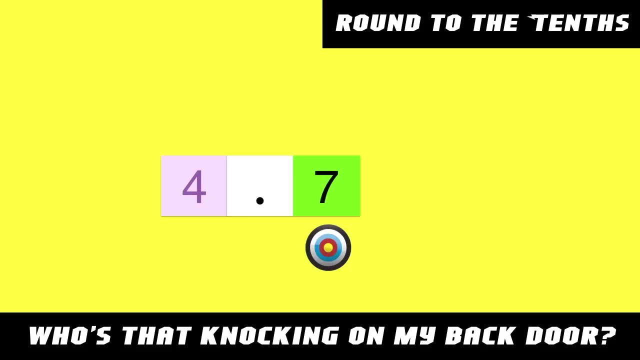 the same. Our new number can be written as four and seven tenths. since the zeros after the seven were not giving us any more information, Our final number, rounded to the tenths, is four and seven tenths. Let's look at another. 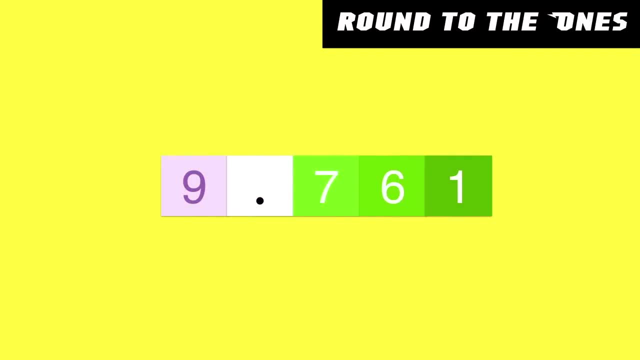 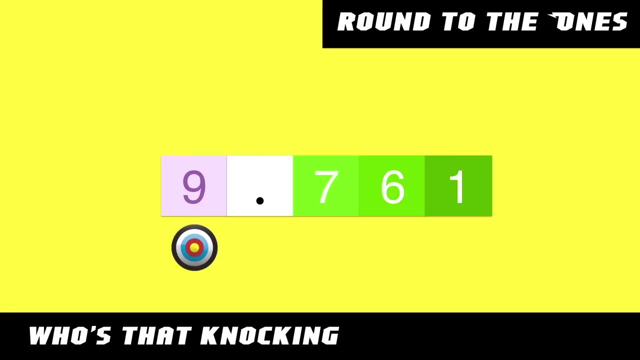 number. This time we are being asked to round to the ones place. Sometimes this is also said as round to the nearest whole number. The ones place becomes our target, Using the rhyme we learned before. who's that knocking on my back door? Seven is knocking on my back. 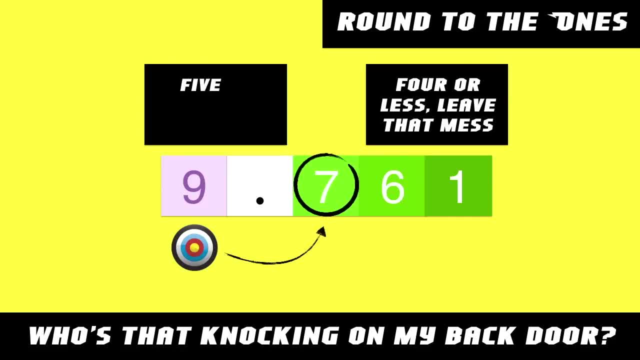 door. Which category does seven fall under? Four or less- leave that mess. or five or more? raise the score. Seven is greater than five, so five or more, raise the score. Remember we're raising or rounding up the target number nine, But wait, how do I round up nine? That's the highest. 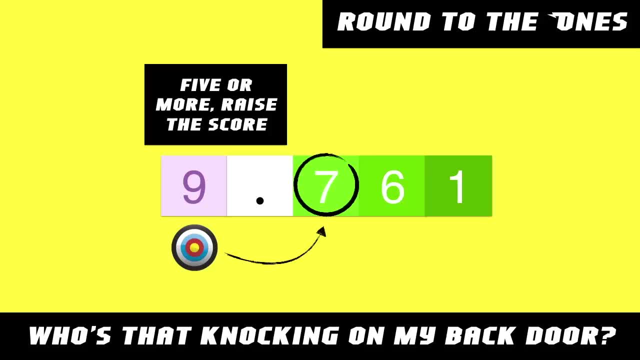 number I can fit in the ones. You're exactly right, but rounding up just means counting up by one. so one more than nine is ten, Which means you will need to add a one in the tens place and a zero in the ones to show ten. All of the numbers to the right of the target.